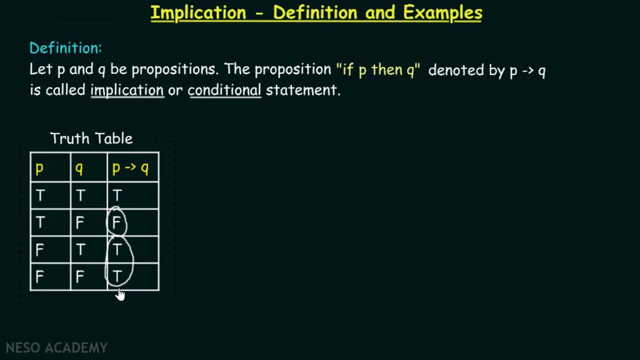 This is most important point to understand. in implication, When P is false, then definitely P implies Q would always be true. We can understand this complicated looking portion with the help of examples. Now let me emphasize one important point related to implication, or conditional statement. 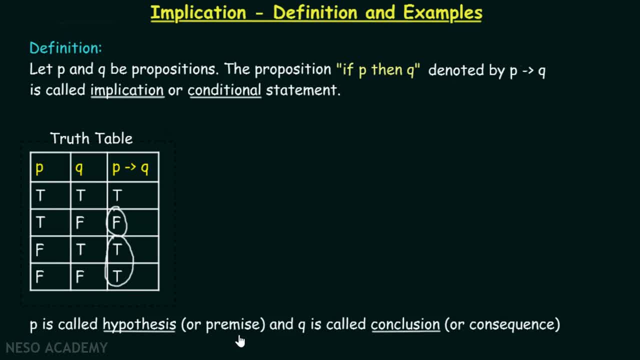 P is called hypothesis or premise and Q is called conclusion or consequence. Here P is called premise and Q is called conclusion. Okay, Now let's consider some examples to better understand the concept of implication. Here is our first example. If you try hard for your exam, 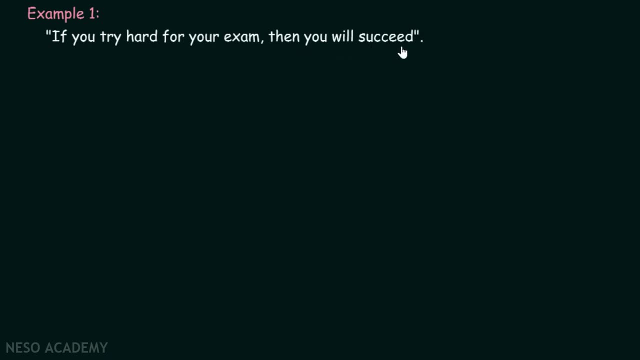 then you will succeed. Now let me ask you one question: Is this particular statement a conditional statement or not? This particular statement is a conditional statement Because we can see that this particular statement is of the form: if P, then Q. Right Now let's see what is P. 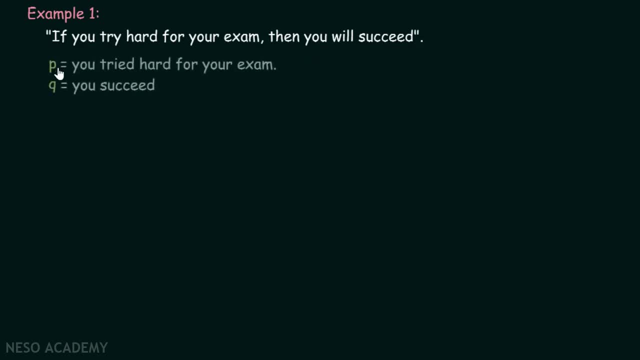 and what is Q in this particular statement Here? P is you tried hard for your exam and Q is you succeed. Okay, In order to understand this particular conditional statement in better details, we will consider four different cases related to this particular statement. Now let's consider our first case. 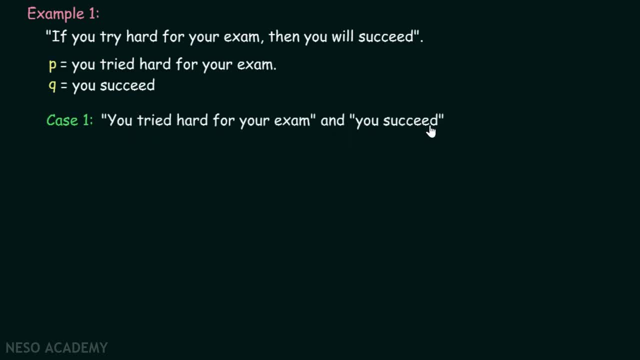 You tried hard for your exam and you succeed. Suppose you tried hard for your exam and finally you succeed as well. This means P is true and Q is also true, Right? This simply means that this whole compound proposition P implies Q would be true. 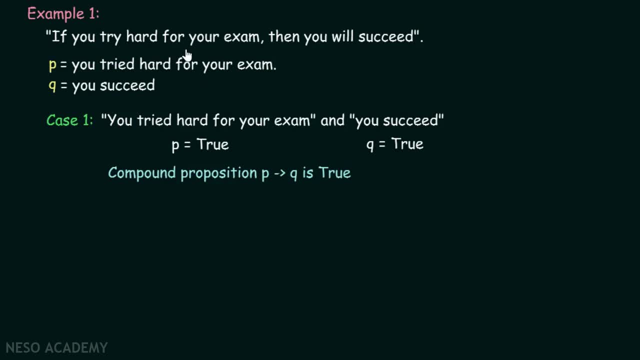 Right, Because you tried hard for your exam and you also succeeded. This simply means that this particular statement is correct. Therefore, according to case one, this compound proposition P implies Q is true. Now let's consider the second case. You tried hard for your exam. 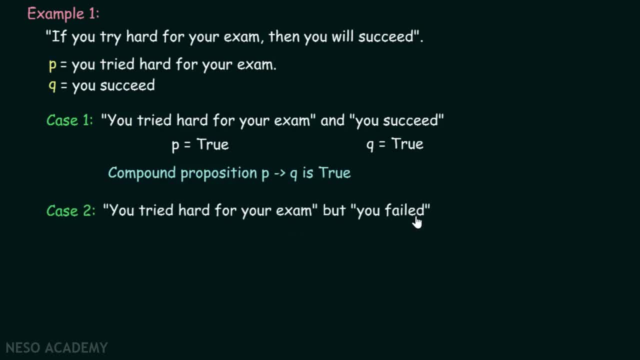 but you failed. That means you tried hard for your exam. You did lot of hard work to prepare for the exam, but finally you failed. This means that P is true and Q is false, And hence the whole compound proposition becomes false. Isn't that so? 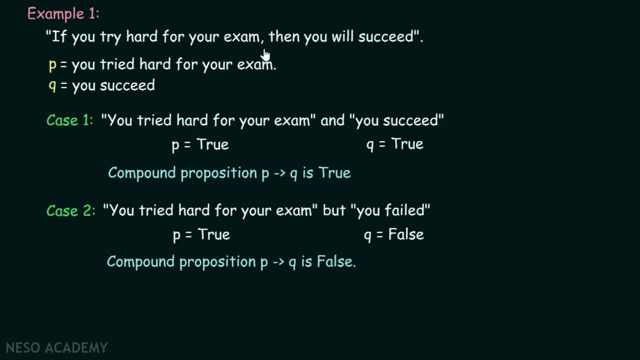 According to this compound proposition, if you try hard for your exam, then you will definitely succeed. But here, you tried hard for the exam, but you eventually failed, Which means that this argument is false. Right Now, let's consider case number three. 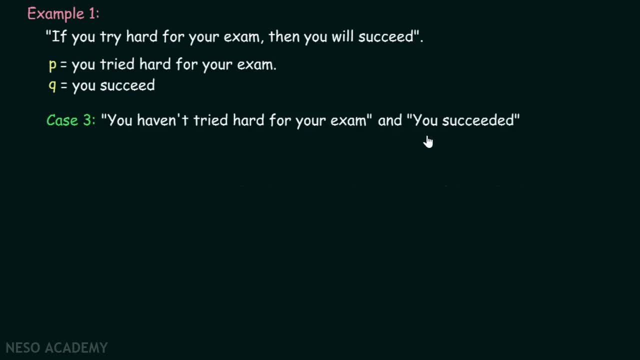 You haven't tried hard for your exam and you succeeded. Now this is one of the most interesting case. we need to understand very carefully Here: P is false. Right This particular proposition: P is false. You haven't tried hard for your exam. 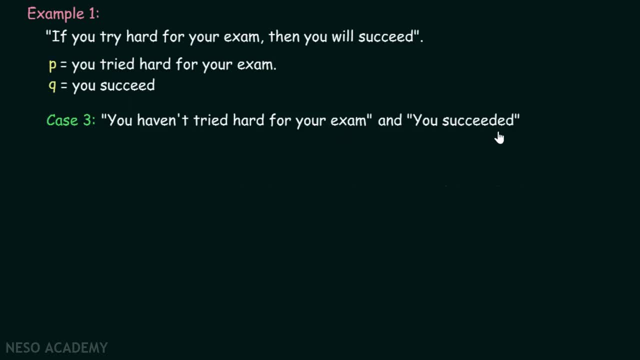 But your luck favors you and you get succeeded. That means P is false and Q is true. According to the truth table, when P is false and Q is true, the compound proposition P implies Q becomes true. But why? Because you can make the compound proposition. 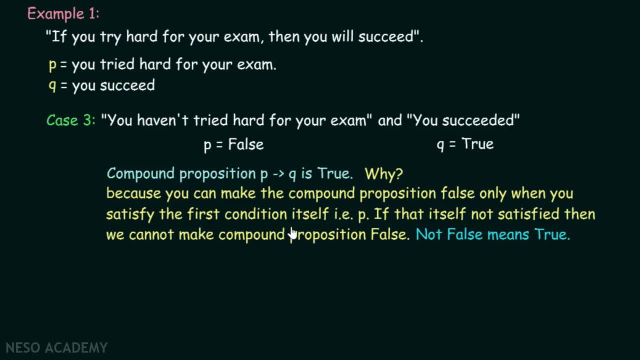 false only when you satisfy the first condition itself, That is, P. Let's try to understand. what does this statement mean? Now? according to this statement, if you try hard for your exam, then you will definitely succeed. Right, But you haven't tried hard for your exam. 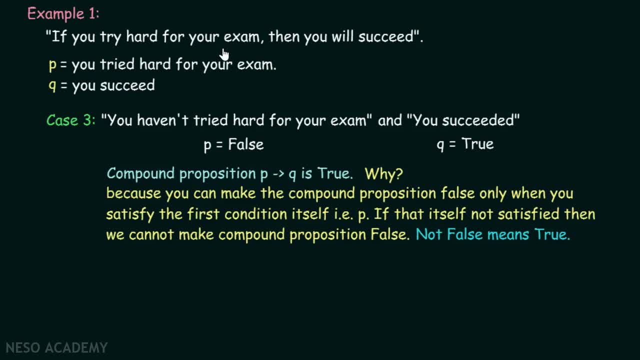 Then how can you come to this conclusion that this particular proposition is false? Try to understand this statement. You can only make this compound proposition false when you make this particular proposition P true. If you satisfy this particular proposition, then only we would be able to. 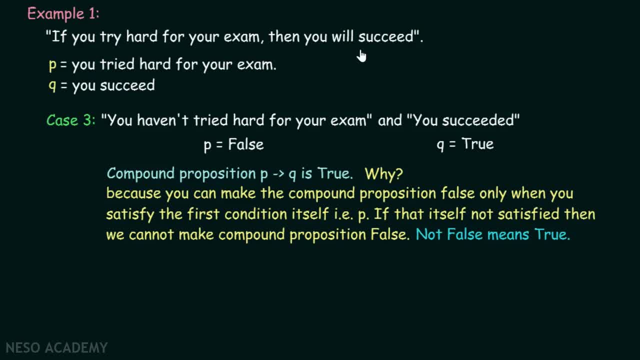 argue about this whole compound proposition. Did you get my point? If that itself is not satisfied, then we cannot make compound proposition false. Right, Not false means true. Therefore we can say that this particular compound proposition is true when P is false. 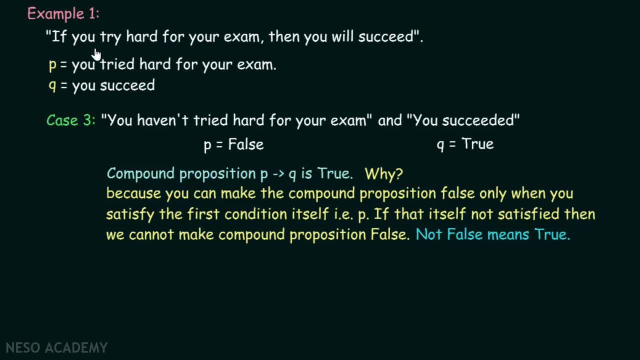 You can only argue about this particular statement when you tried hard for your exam. If you haven't tried hard for your exam, then how can you argue about this particular statement? You cannot make this statement false. Let's consider the another case. You haven't tried hard for your exam. 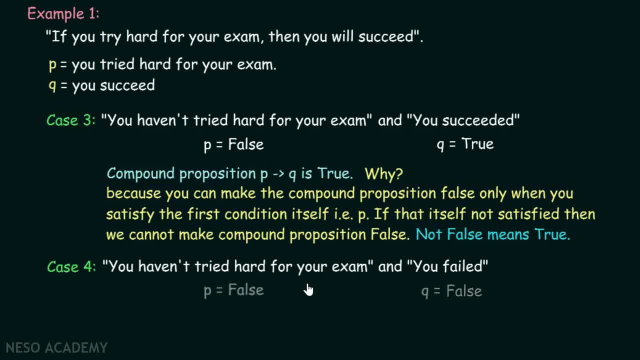 and you failed. Now we know that P is false and Q is false. Because P is false, we would not be able to make this particular proposition false, Isn't that? so This proposition can be made false when you tried hard for your exam. 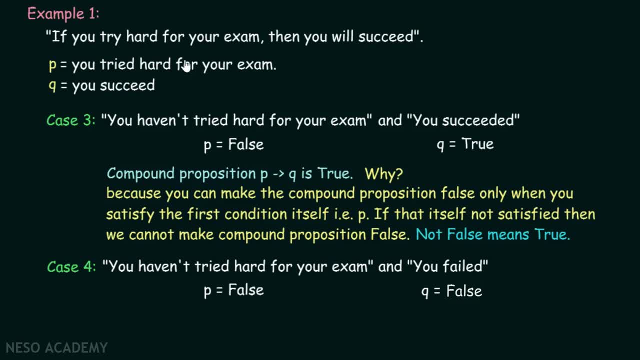 and you eventually failed, But here you haven't tried hard for your exam. If you haven't tried hard for your exam, then you are out of this statement and you would not be able to make this statement false, Right, Therefore, this compound. 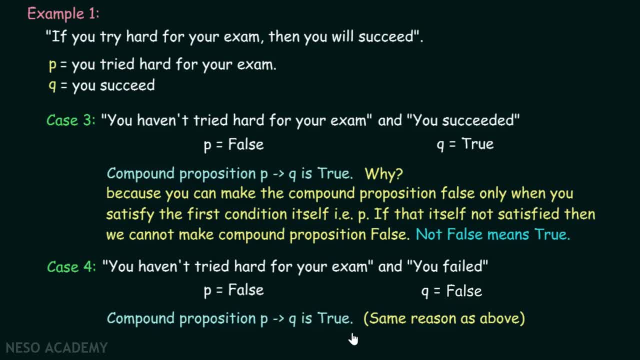 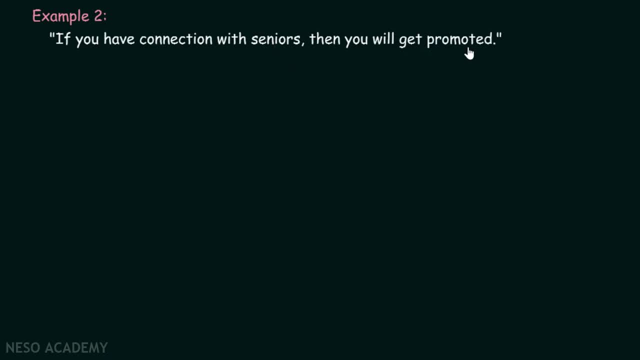 proposition is true. Now let's consider one more example to cement this concept: If you have connection with seniors, then you will get promoted. According to this statement, if you have connection with seniors, then you will get promotion. Suppose you have connection with seniors. 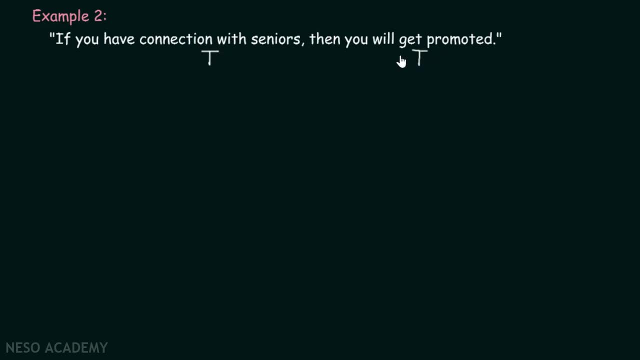 and suppose you will get promoted as well, then definitely this statement would be true. Right, This whole compound proposition would be true. But if suppose you have connection with seniors and you will not get promoted, then you will feel like cheated. I do have connection with seniors. 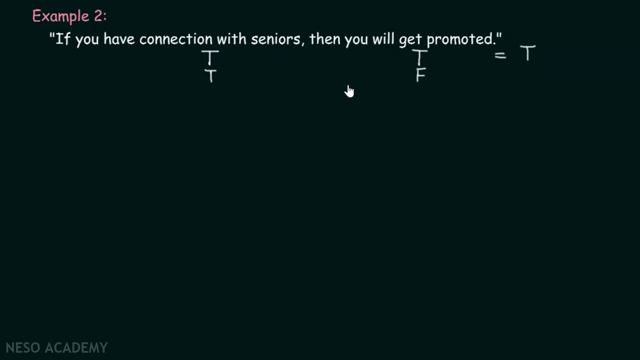 but I am not getting promoted. Then you come up with this conclusion that this particular statement is false. Isn't that so? But if you have no connection with seniors, it doesn't matter, you will get promoted or not. You cannot argue about this. 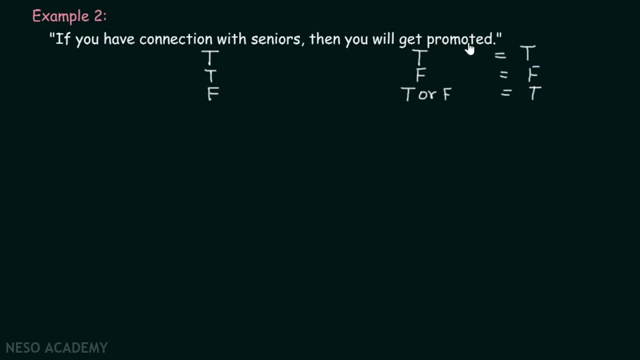 particular statement that this statement is false. Let's consider one more example. If you get 100% marks on the final exam, then you will be awarded a trophy. If suppose this is true and if suppose this is false, then you feel like cheated. 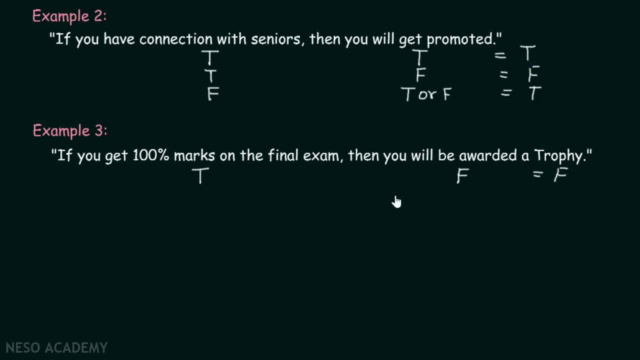 Isn't that so, Then this particular compound proposition would be false. But if you won't get 100% marks, then there is no point of considering this whole compound proposition. This particular compound proposition remains true. This is very simple to understand. 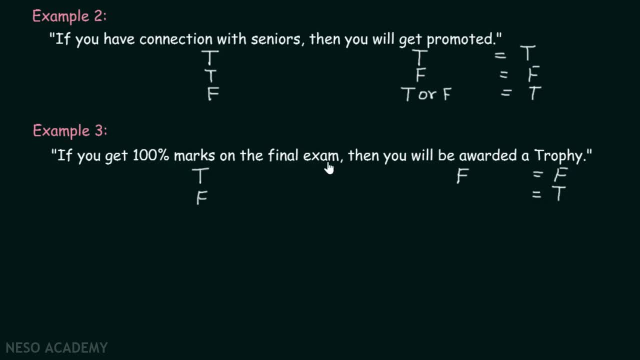 If you won't get 100% marks on the final exam, then how can you ask for a trophy? If you get 100% marks, then definitely you can demand for a trophy. If you get 100% marks and you are not getting a trophy, 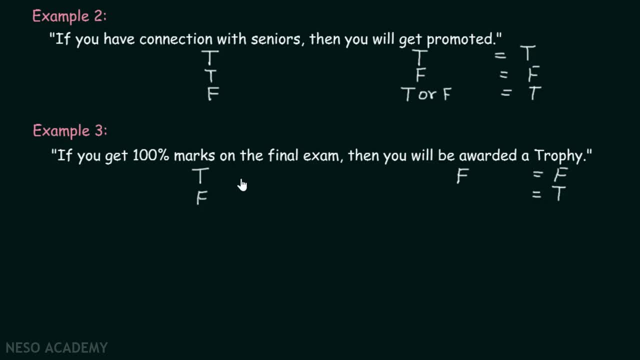 then definitely this statement is false. But if you won't get 100% marks, then you cannot demand for a trophy. You may get a trophy or you may not get a trophy, But you cannot say that this particular statement is false If you won't get 100% marks.